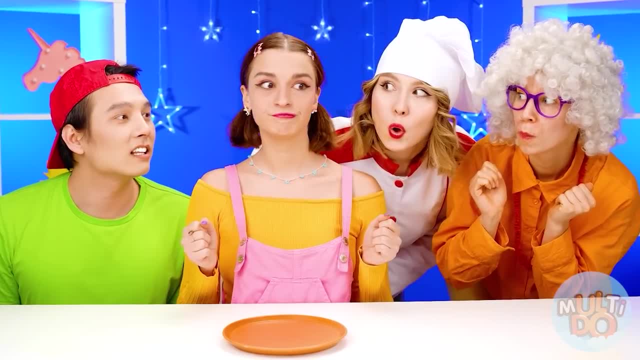 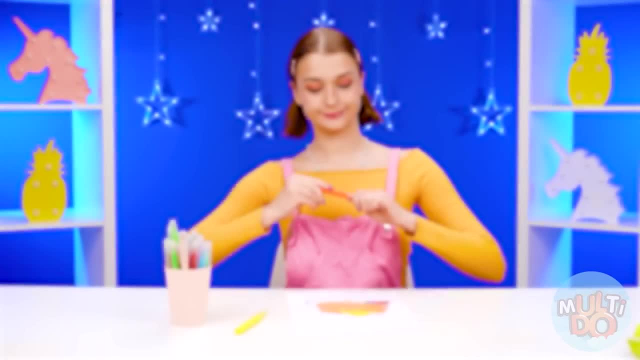 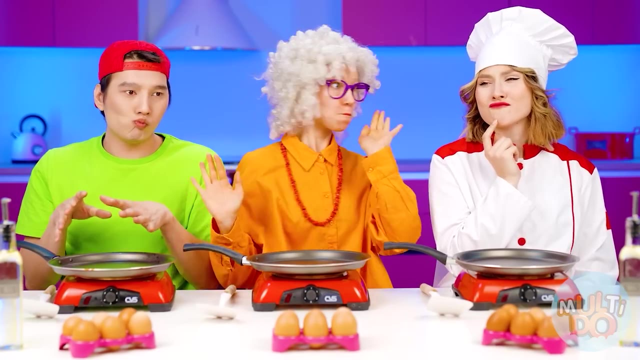 What took you so long? I'm hungry, So I propose a challenge. Welcome to Multidoo. We'll start with a simple one: Cook me some delicious pancakes. Pancakes- I can do that. I've made so many pancakes in my life, I know their recipe by heart. 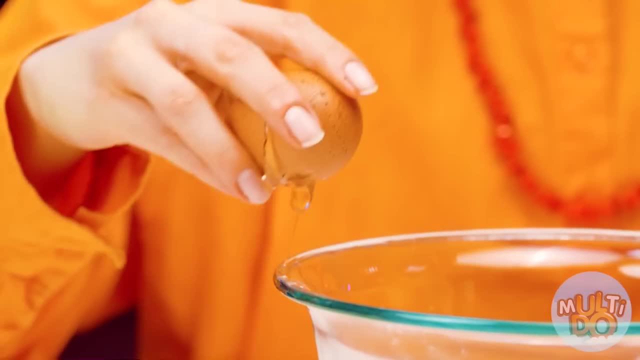 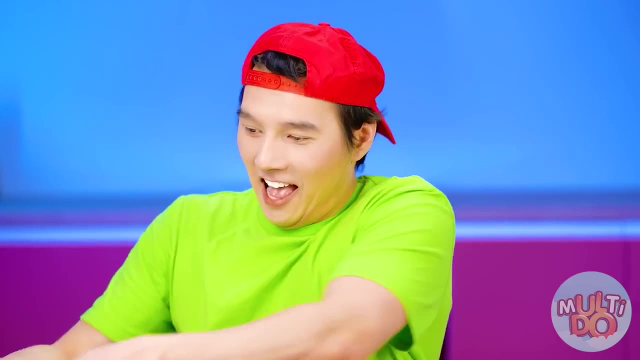 First you need to mix flour with milk, Then break the egg into the resulting mixture. Zach, what are you waiting for? Repeat after me. How do you say you need to do this? I have a deep plate. The only thing left is poor flour there. 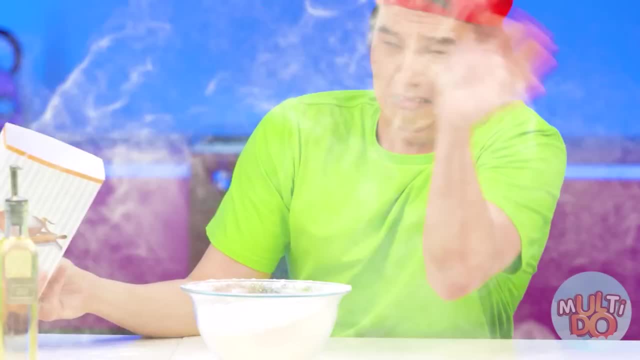 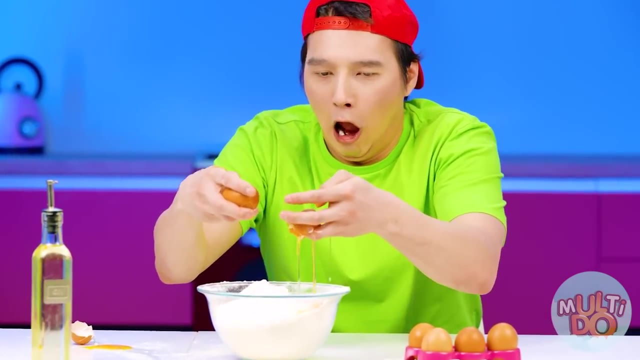 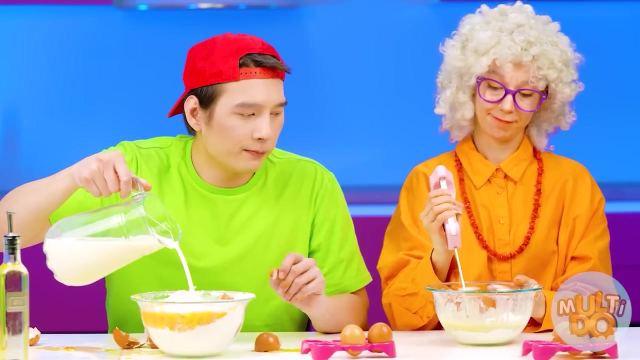 And the more the better. Ugh Yeah, it's not easy to cope with flour. Next come the eggs. You also need to be careful with them, And we must not forget about the milk. Grandma taught it that way. Whoa Grandma, Yes, you have a full-fledged doll ready. 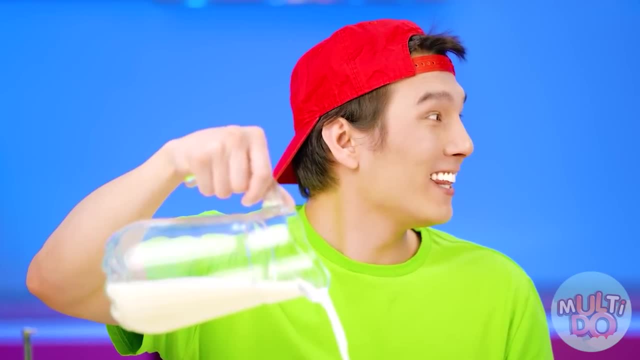 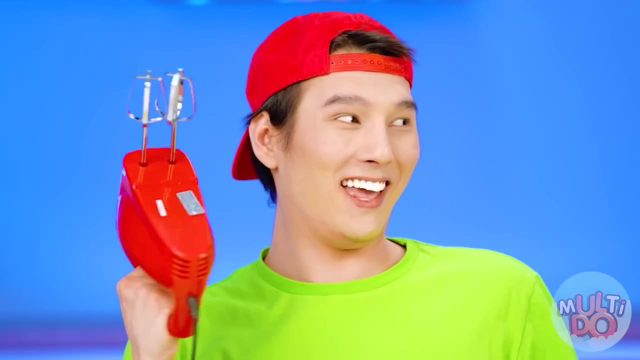 Yes, yes, There will be pancakes soon. Dammit, What have I done, Granny? it's all your fault. I was distracted by you and accidentally poured my doll. But never mind. I think after I shake it up, everything will be okay. 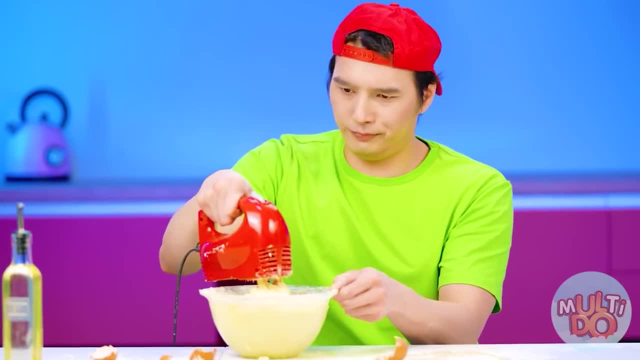 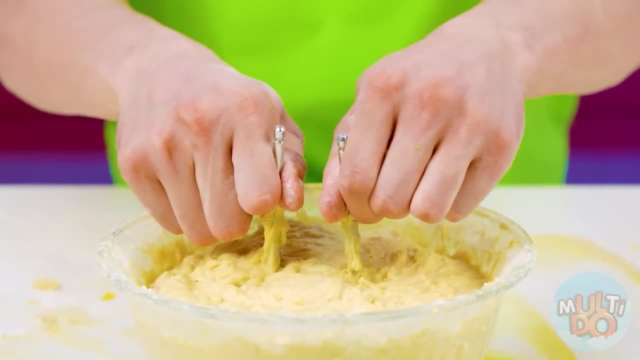 Strange. Uh, this stupid mixer is just stuck. Come on, get out of there. Uh, where are the mixer nozzles? Oh no, How do I get them out? Ugh, Apparently they have settled in my dough forever. 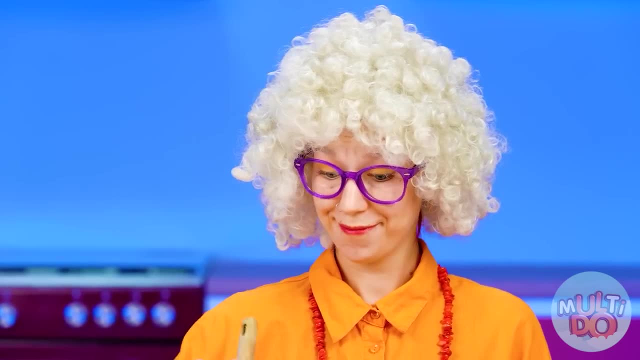 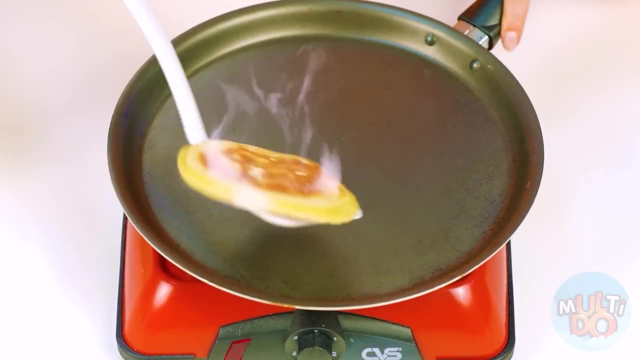 Yeah, Zach, You're a lousy cook. We'll have to cook the most delicious pancakes ourselves. I don't have any competitors anyway. Just look at this beauty, So beautiful. Of course, these pancakes need to be poured with maple syrup. 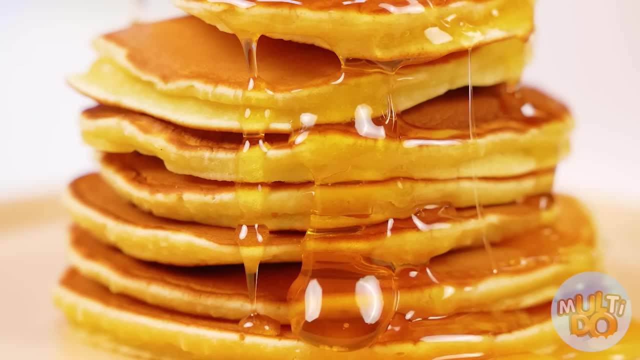 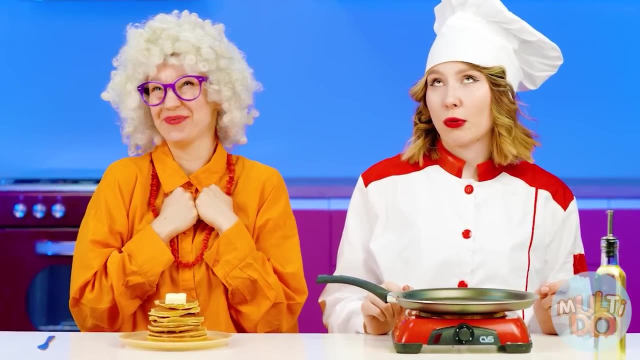 Of course these pancakes need to be poured with maple syrup. Of course these pancakes need to be poured with maple syrup, So they will become even tastier. A piece of butter wouldn't hurt either. Granny turned out, of course not bad, but too boring. 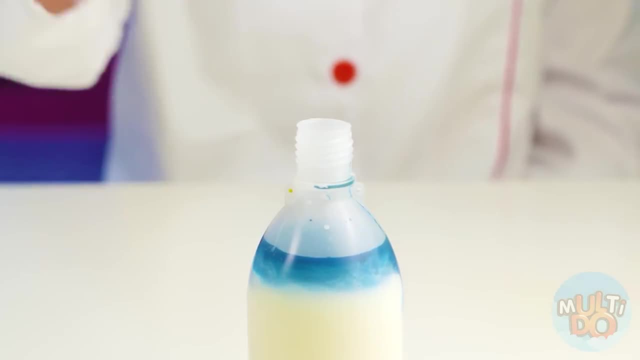 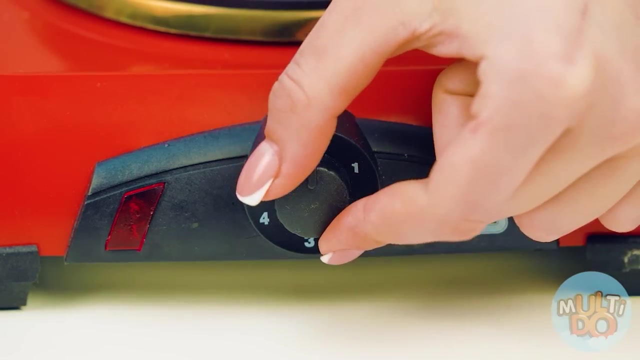 Why not make pancakes also colorful, So it'll be more interesting to eat them? Wow, Beauty, The dough is ready, Let's cook. My pancakes are in the oven. My pancakes are in the oven. My pancakes are in the oven. 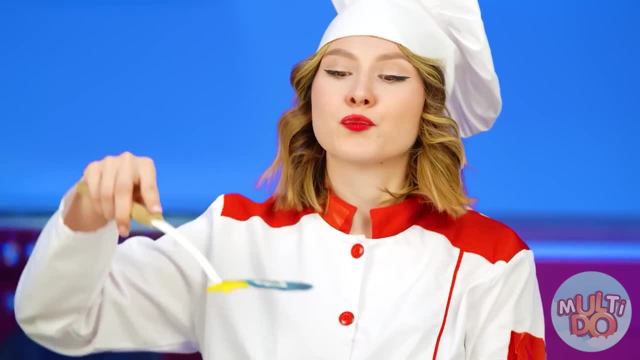 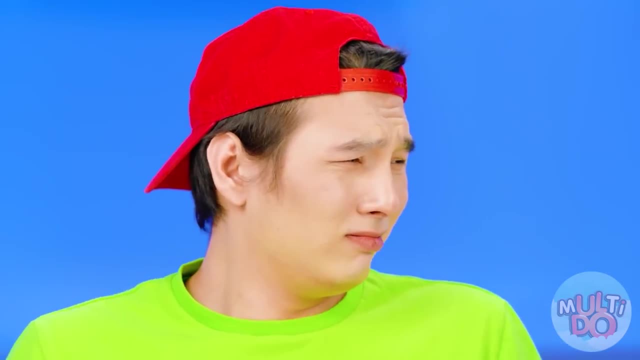 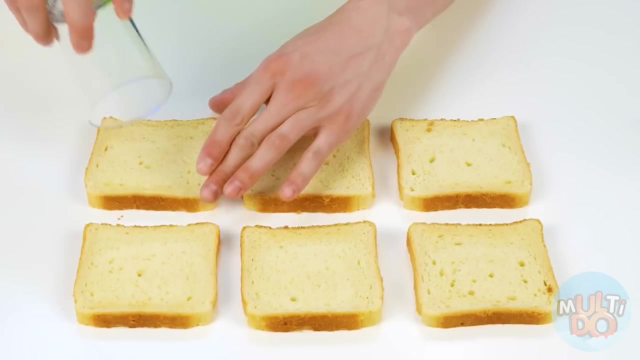 Let's flip it Just a little more on the other side And ready. Well, everyone gets such beautiful pancakes. What should I do? That's right. Why cook pancakes from Da? You can just take the finished one. For example, cut out a circle of bread with the help of cups. 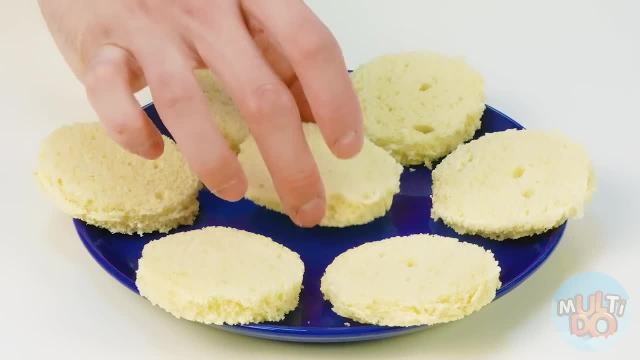 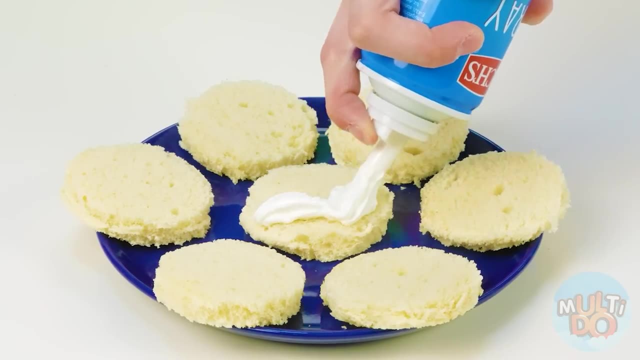 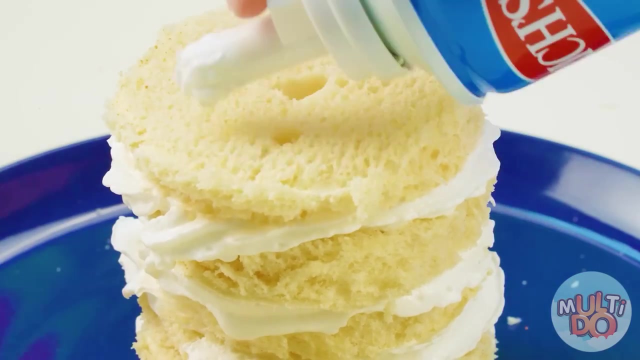 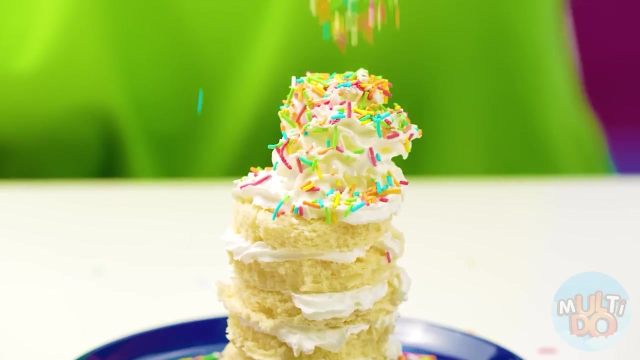 To make them tastier, you need just sprinkles and whipped cream, And if you add a little bright sprinkles, my brand's pancakes will become even tastier. Look, It's almost ready. The last gesture… Look at this beauty. 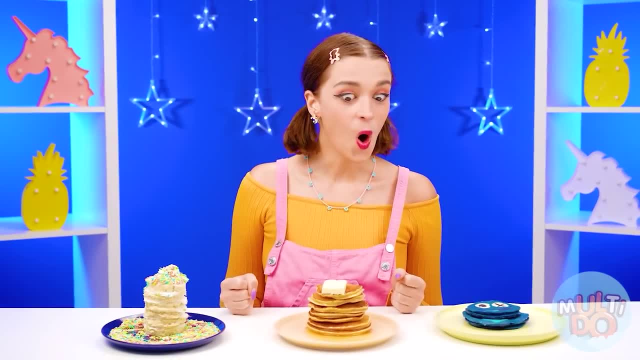 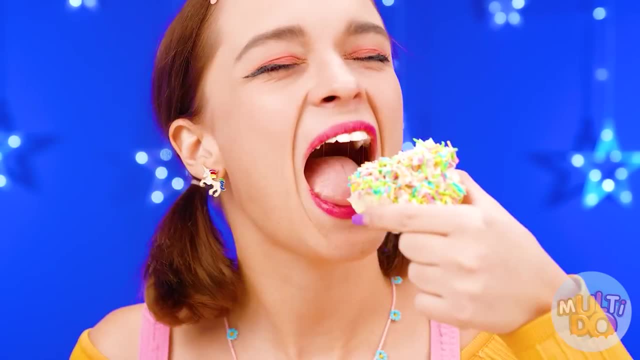 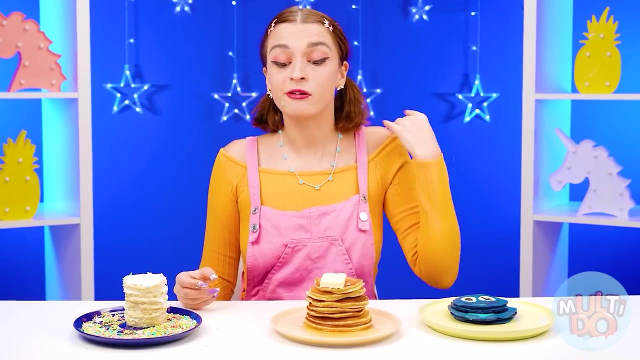 Kate, it's time to pick a winner. Wow, I didn't expect such a variety of pancakes. Let's start with Zack. I hope this pancake won't disappoint me, Although they look quite strange. But sprinkles and cream are good. 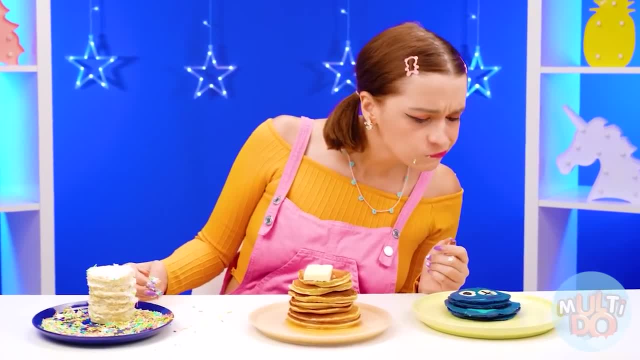 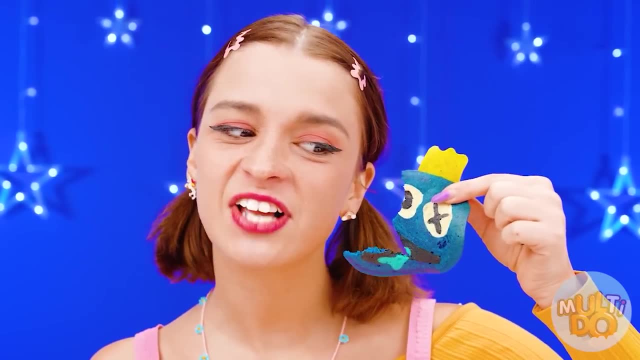 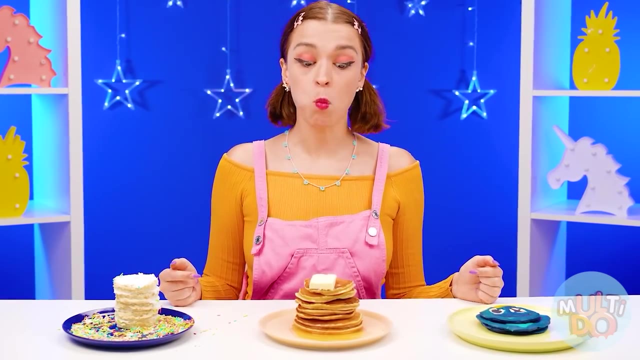 Well, let's move on. Who are these blue freaks? Original, But are they delicious? Ooh, I really like it. This time they definitely tried for me. Well, the only one left is from Grandma. Grandma, don't let me down. 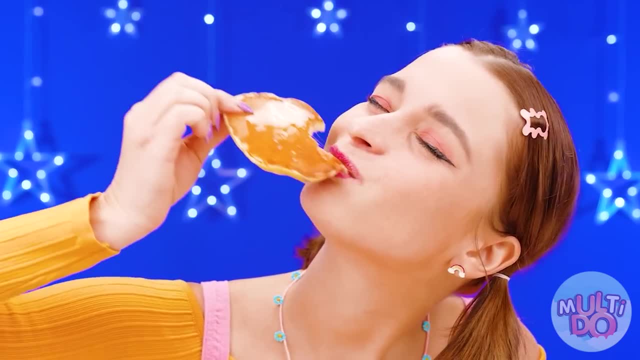 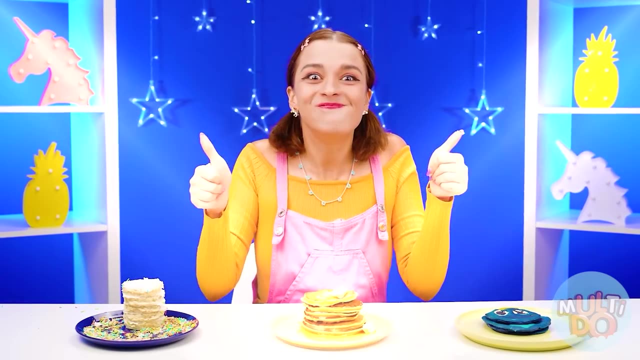 Mmm, so gorgeous. Oh, a taste of my childhood. Grandma, you know best how to make delicious pancakes, so the victory in this round goes to you. Oh hooray, don't worry, someday you will be lucky too. 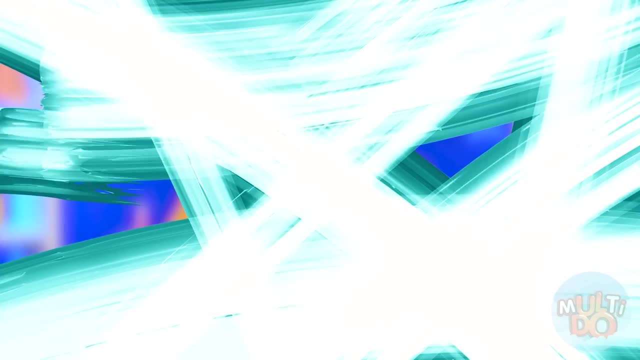 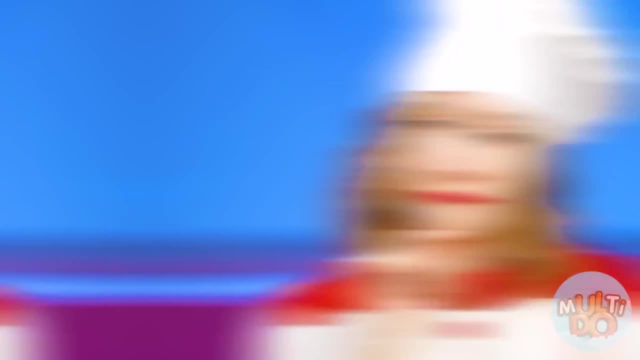 Oh, look at this. It's so cute. She's even cooking for a family. Sweet Cool. Are you ready for the second round? Then make some delicious hot chocolate for me right now. We'll be done Easy. Well, everyone is chatting, I, as the smartest, enjoy Nutella. 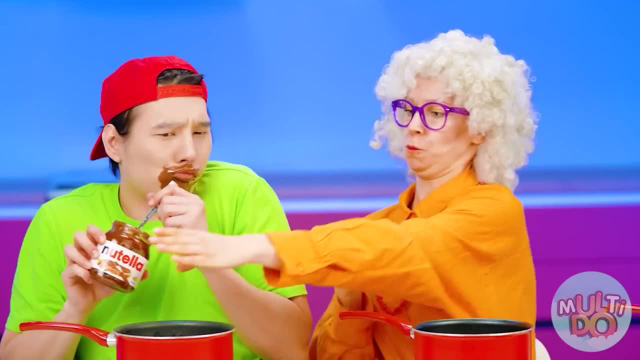 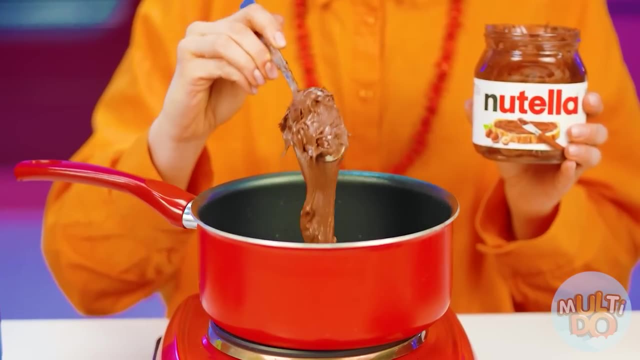 Zack, aren't you ashamed of yourself? I need this Nutella to make hot chocolate for Kate. I plan to win this round too. To do this, I need to stir the Nutella with milk… Then put the sweetened cream on top. 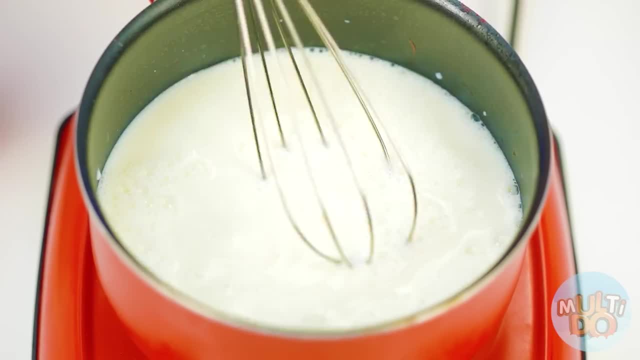 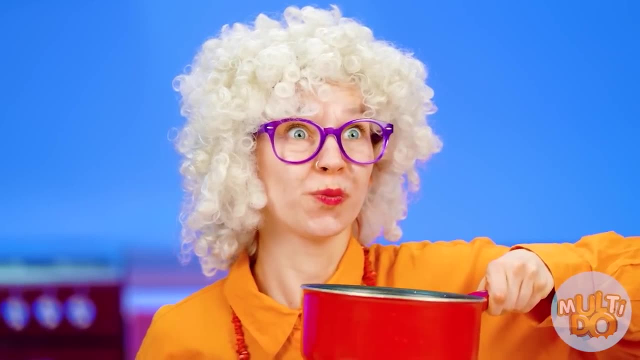 And the original Museum cake is ready. What do you need to do to make it? Let's start with the dark chocolate cake. I want to make enterprise cookies. Put this mixture on the fire And, of course, stir it well. Mmm, smells delicious. 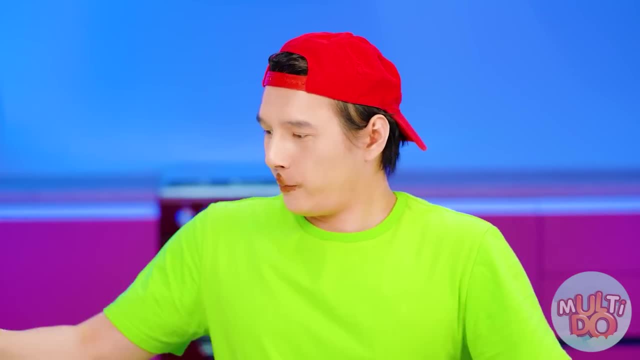 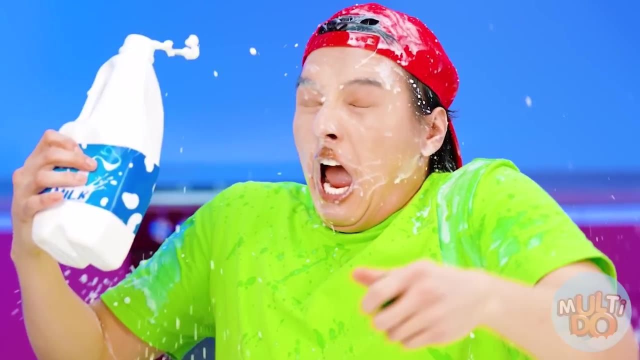 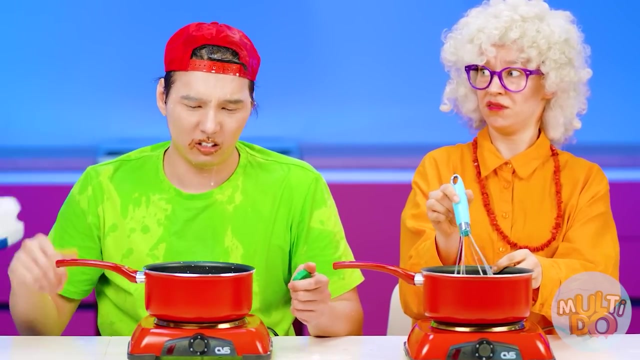 Oh yeah, the smell is amazing. It's time for me to start cooking, But the milk won't open. Ugh, I'll finish you off anyway. Oh no, I'm covered in milk myself. I definitely need to win So that sacrifices were not in vain. 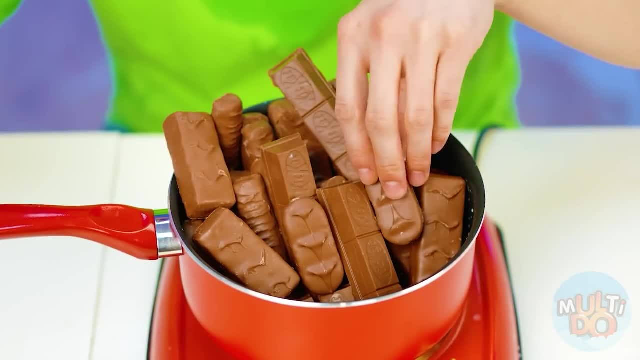 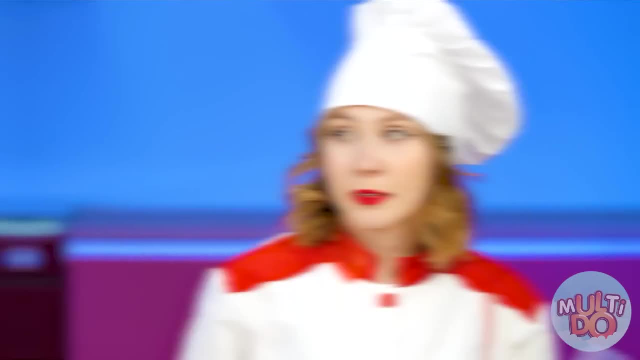 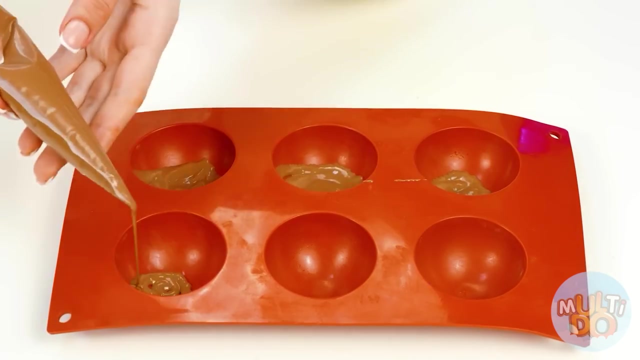 To do this, I use the favorite chocolates of all people on the planet. I will definitely not lose face with them. Watch and learn. Hot chocolate is the last century. Today, chocolate is served separately because it looks more beautiful this way And it also is much tastier. 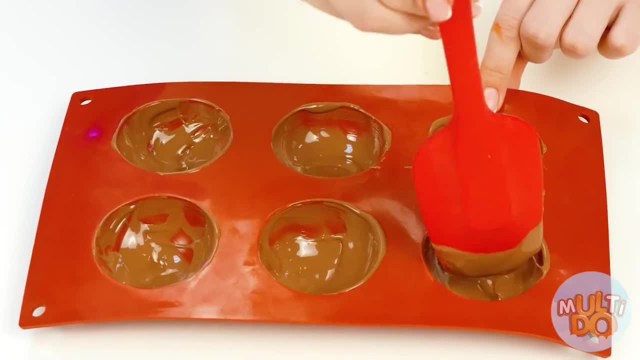 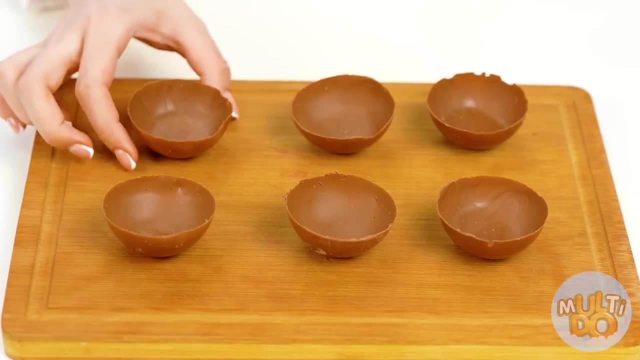 I just know an excellent form from serving it. It just needs to be smeared in a special shape. This way, there are going to be half spheres, And then I'll put them together to make a ball. I'll pour cocoa inside so it will taste even better. 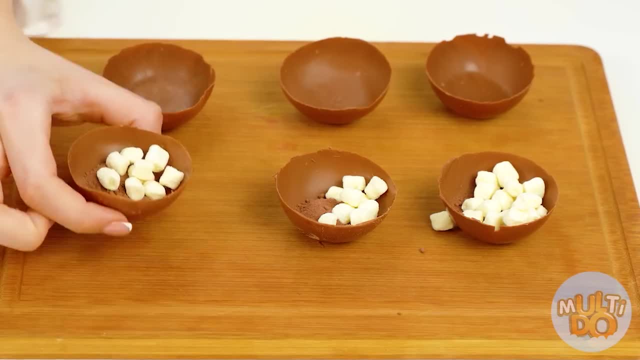 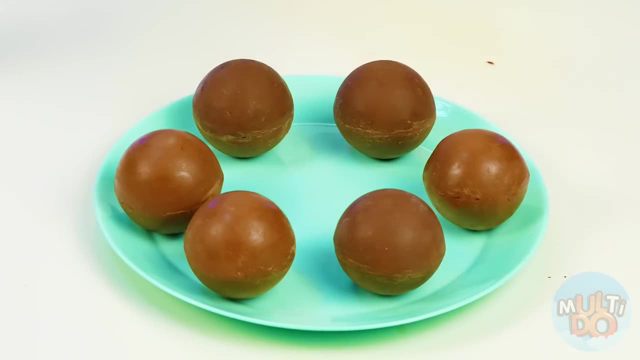 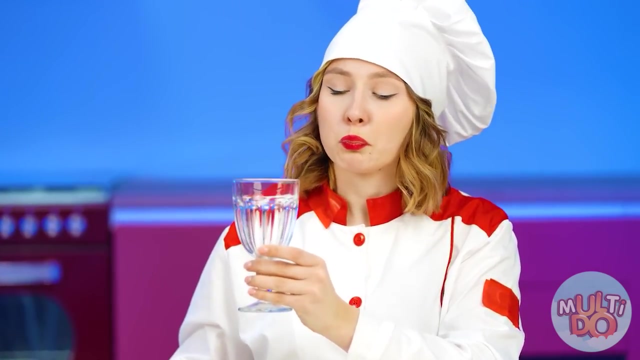 And some marshmallows too. And now just close it, Voila, And I'm going to put more chocolate on top. Just perfect, Now you can pour hot milk into a glass. It is enough to throw one ball into it as it. 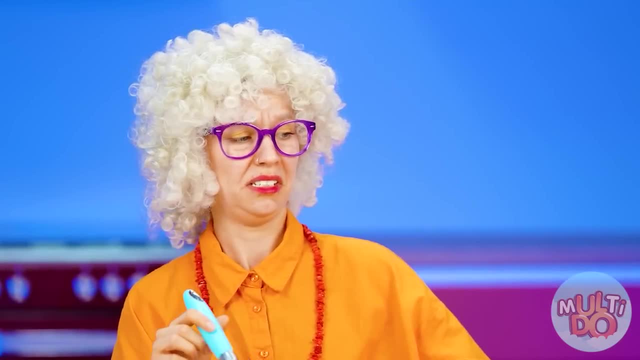 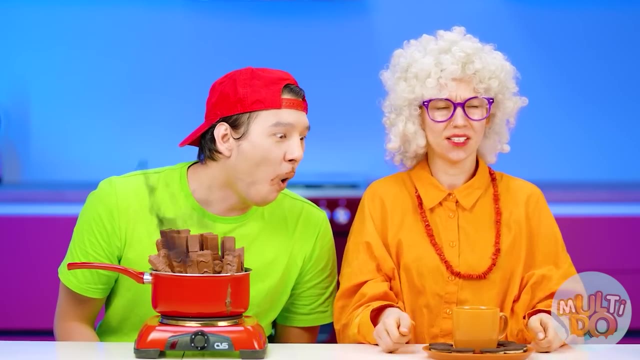 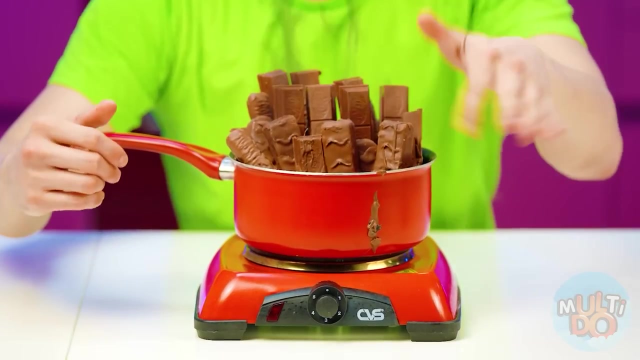 immediately becomes chocolate. Oh, so difficult. My granddaughter loves homemade cocoa and hot chocolate. I like it too. What is this smell? Ah, Zach, your hot chocolate is burning. Oh no, I'm going to turn it off. Why is chocolate so hard? 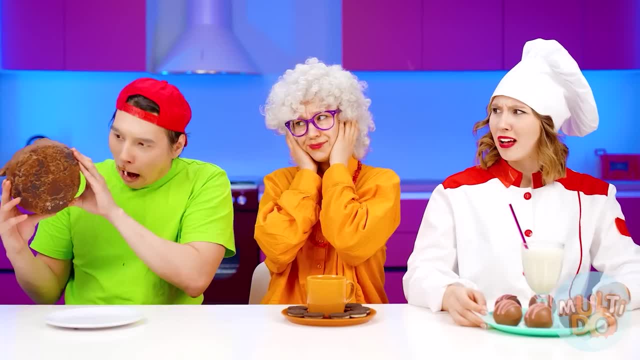 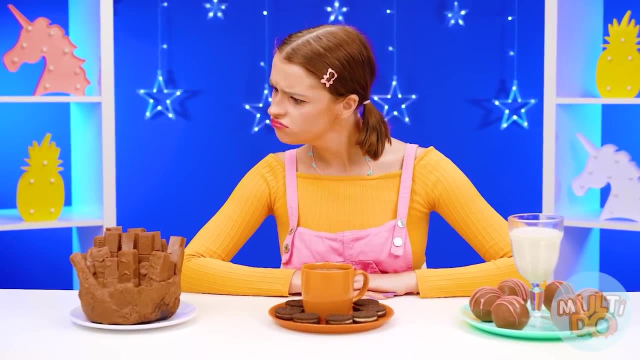 Didn't I cook anything, Oh no, Well, let's pretend that I planned it. Chocolate sculpture, Well, well, well, Zach. I'm sorry, Zach, what did you do? It doesn't really look like cocoa or hot chocolate. 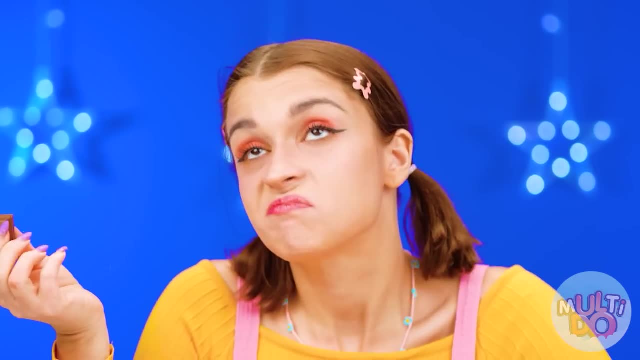 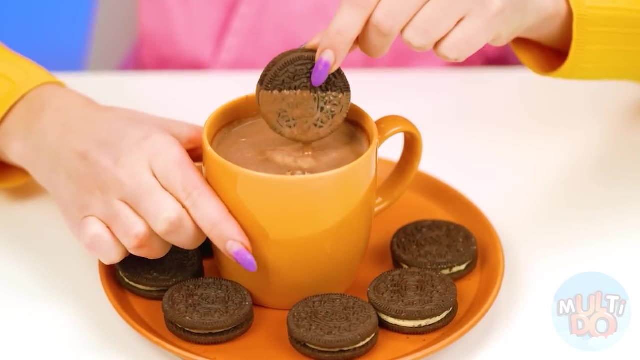 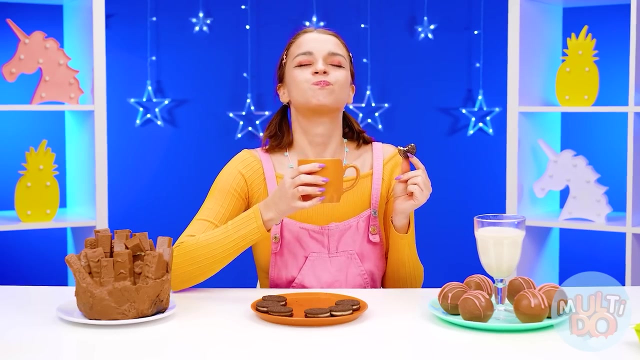 Big deal. It's just a bunch of chocolate bars. That won't do. Let's see what my beloved granny has prepared for me: Mmm. homemade cocoa, Yummy, Also with cookies, Mmm, so good. The only thing left is to try what a miracle Chef Tina has prepared. 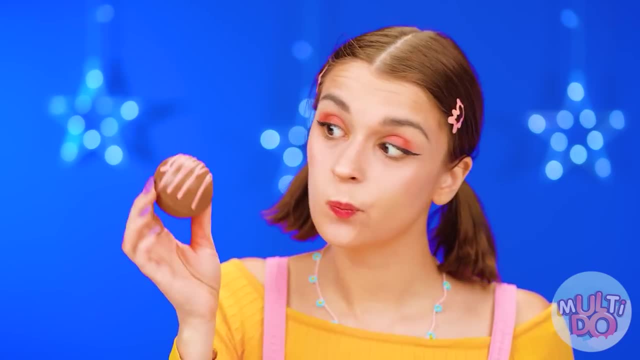 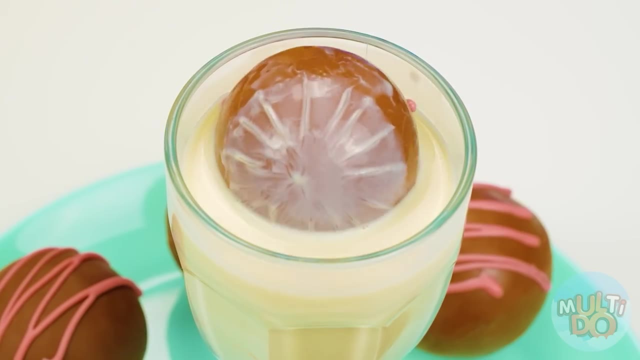 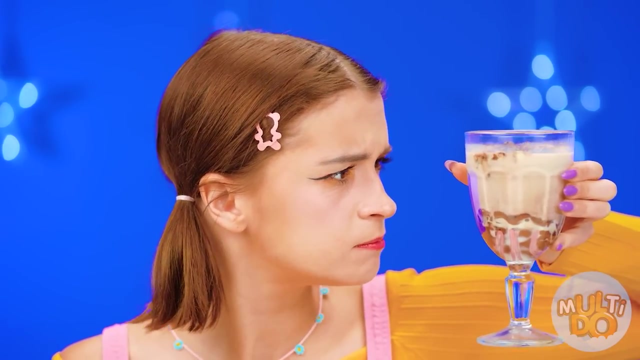 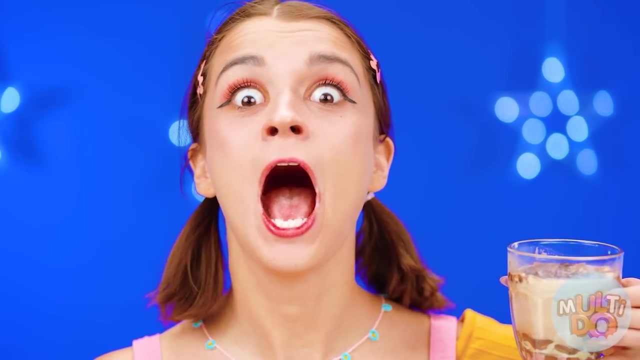 The pitch, of course, is much more interesting than the rest. Whoa, I think I got it. Her hot chocolate is something incredible. Ooh, look how it melts- So magical. Is it really chocolate? Let's try. Mmm, it's just something incredible. 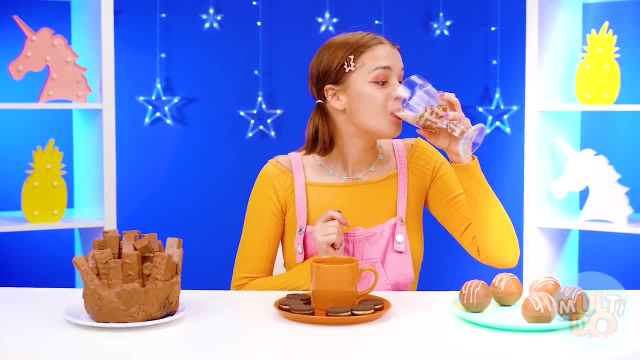 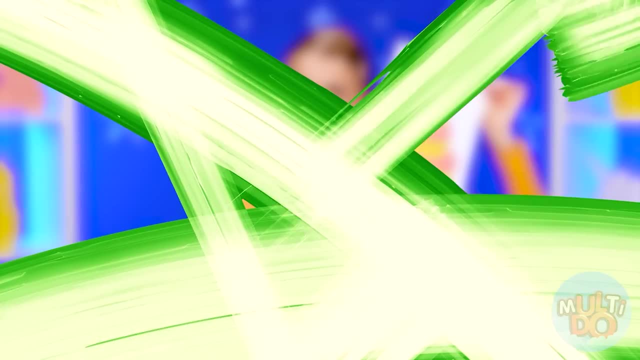 The winner of this round is obvious. Tina, you're becoming one of us. Let's go. I'm the only one. Ugh obvious. After all, I'm the only professional here. Now. I want a cake, Big and delicious. 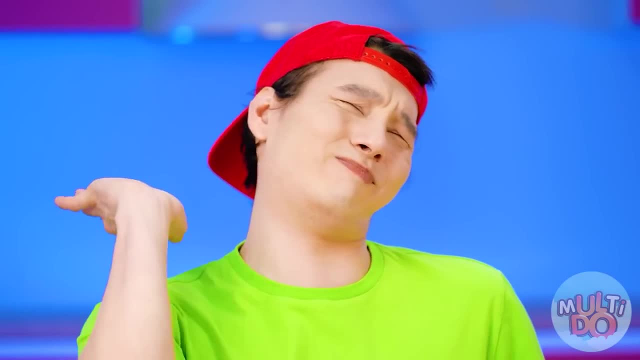 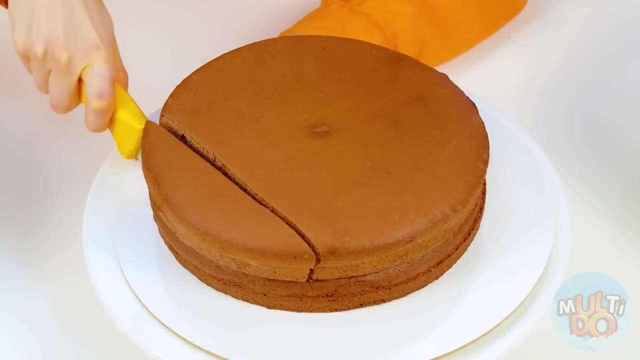 I can cook cakes very well. Easy, I can definitely handle it. It's good that grandma knows her granddaughter's taste. I will be able to cook exactly the cake that Kate loves the most, And I will make it in the shape of a heart. 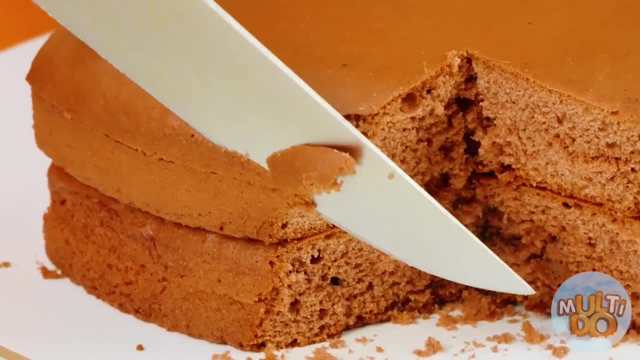 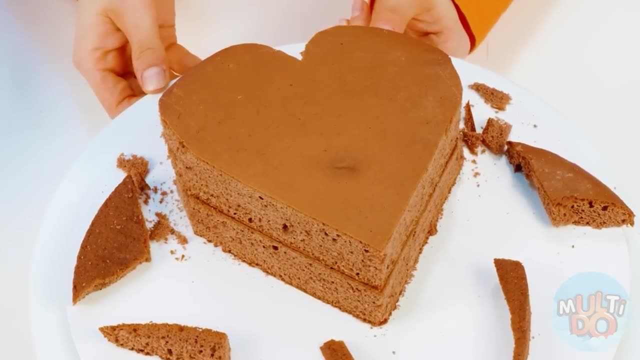 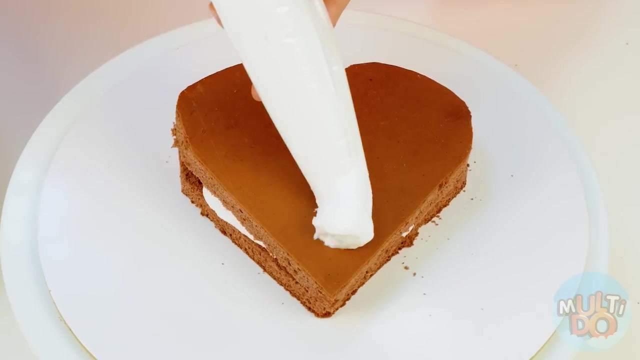 I'm so excited I'm going to make her a heart so that she also knows that I love her. Just like that, So cute. The layers need to be thoroughly smeared with cream so they won't stick together. The more you've got the cream, the more delicious the cake will turn out. 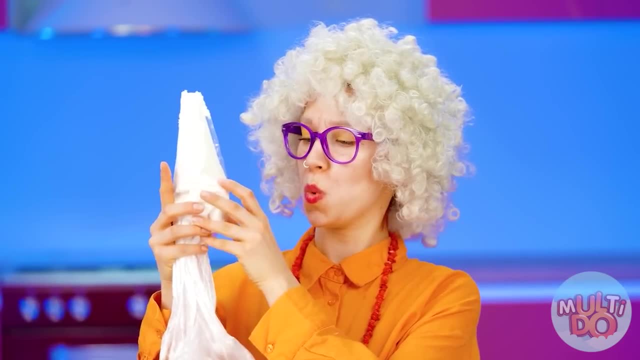 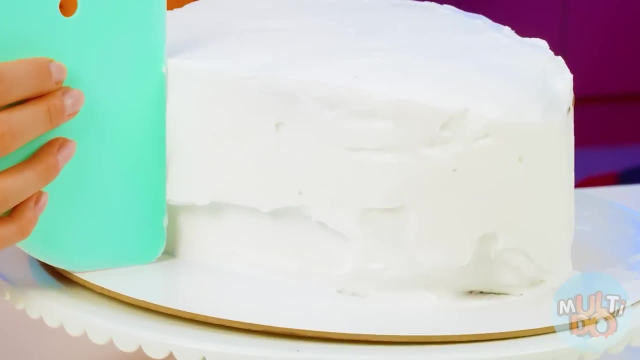 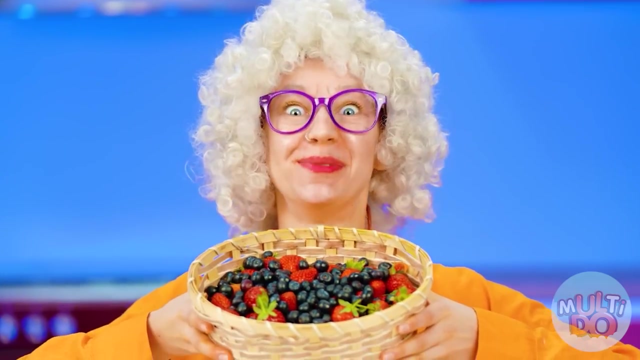 Therefore, you need to smear every millimeter of the cake with cream. And now I'll just even the sides from the cake, the sides from the cake Ready, So good. Now there are no better decorations for a cake than fresh berries. 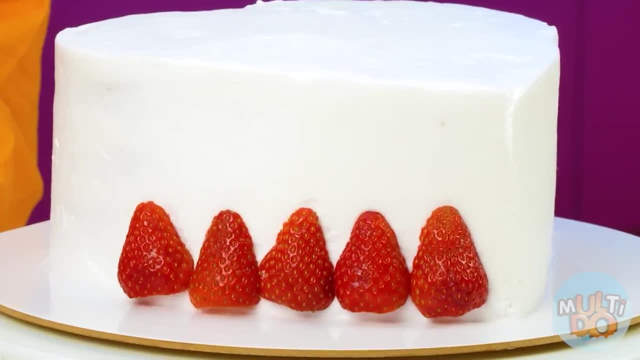 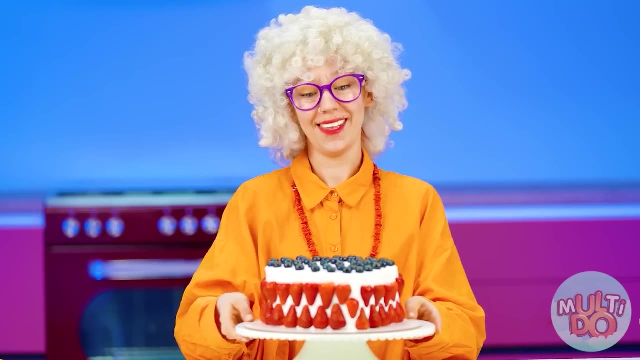 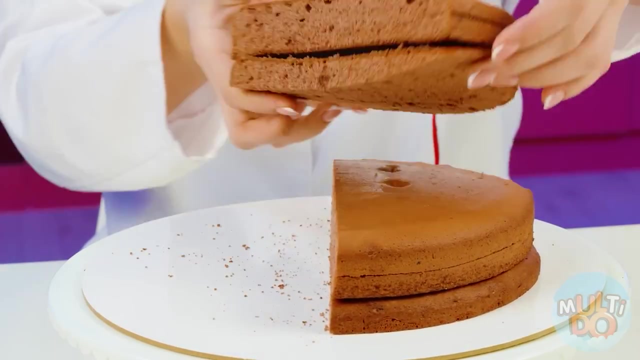 You need to cut off the extra leaves from them and combine berries with the cake. Berries will give the cake sophistication and, of course, a pleasant taste. How do you like my creation? It's corny somehow. Now I will show you how to cook a delicious and great original cake. 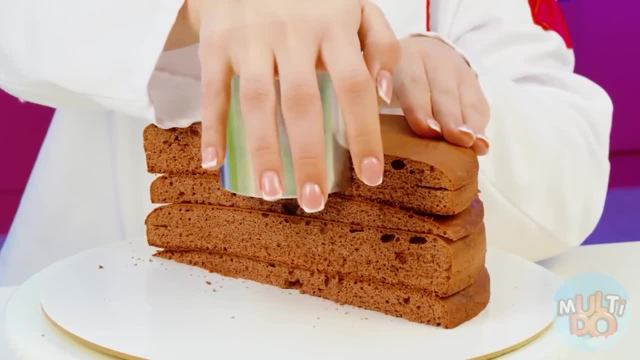 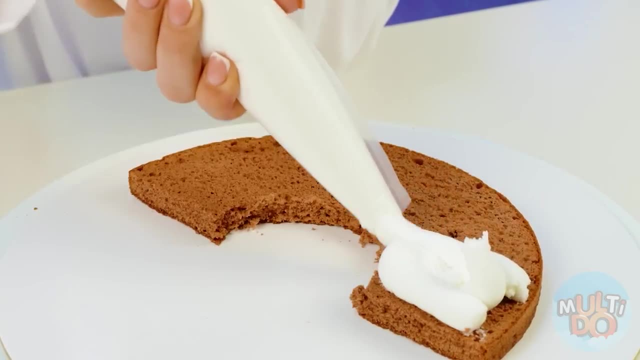 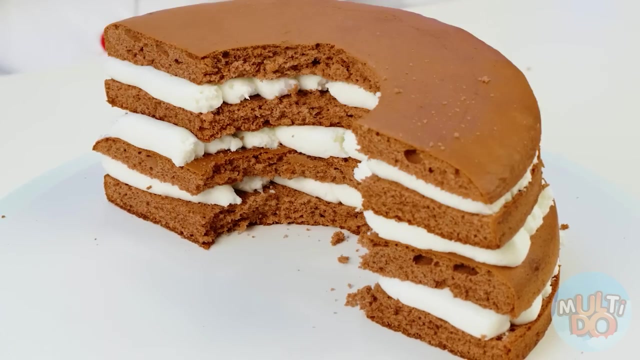 First, the cakes should be divided into two parts, after which a piece should be cut out of a cake Ready. After that, you just need to repeat. after grandma, but not for long. After each layer is covered with cream, time to flip and design it. 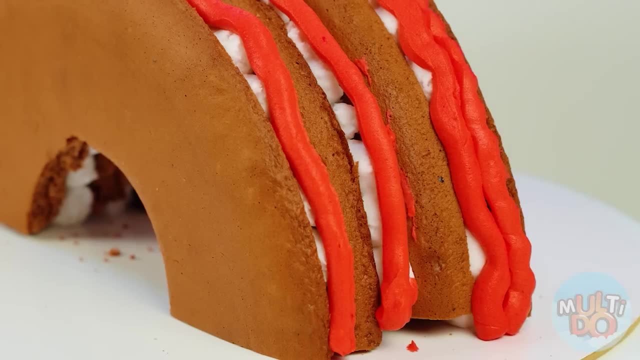 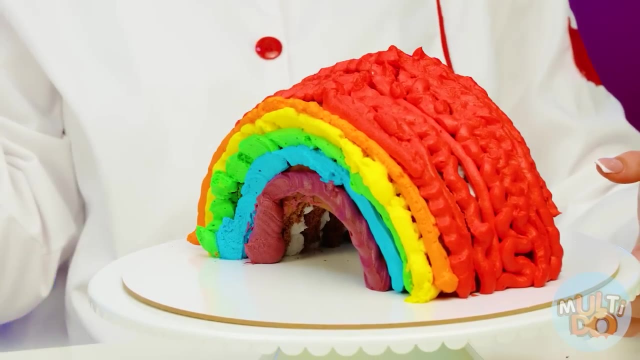 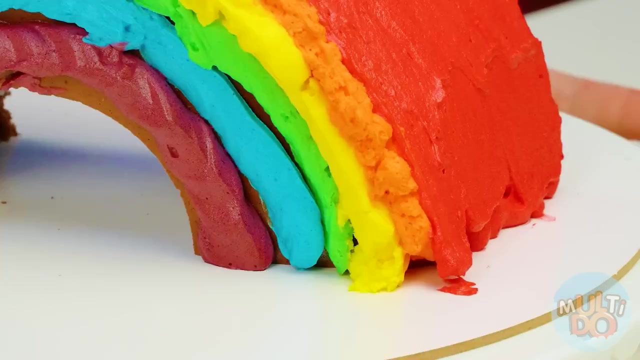 Perfect, The base of the future rainbow is ready. Then we just need to decorate it with the right colors. I'm sure Kate hasn't tried a rainbow cake yet. Well, almost everything is ready. The only thing left is to smooth the cream and add some details. 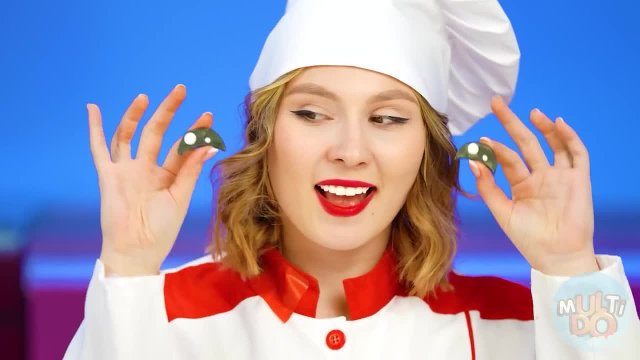 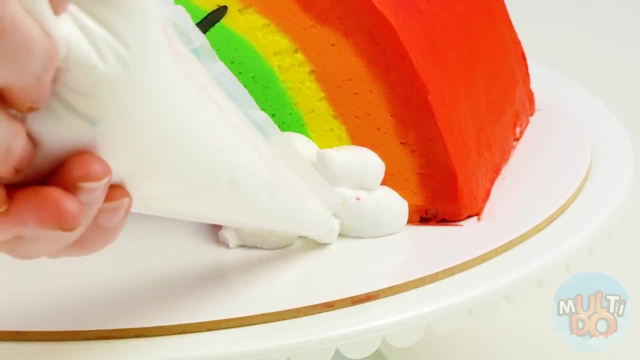 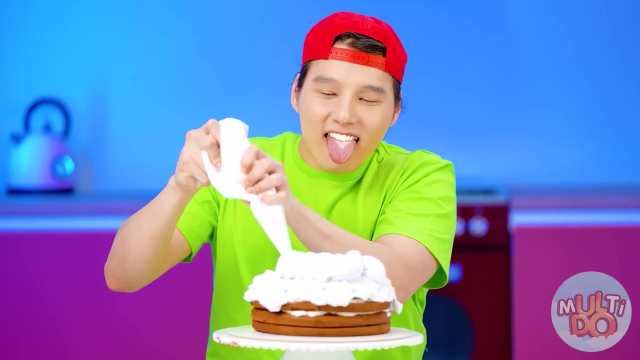 Perfect, And now we can just add some details. A rainbow with a face will be much more cute, And you can also finish off with drawing some clouds. Another one of my masterpieces are ready. Why bother so much? It's a cake. 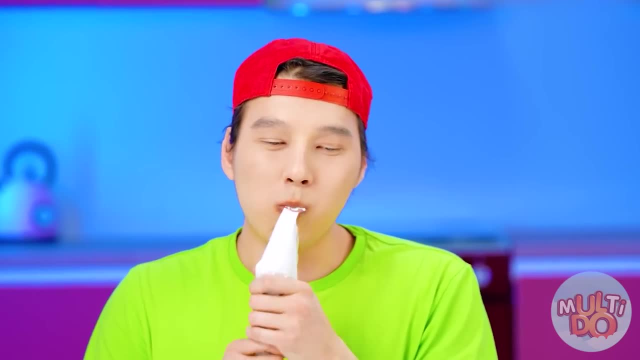 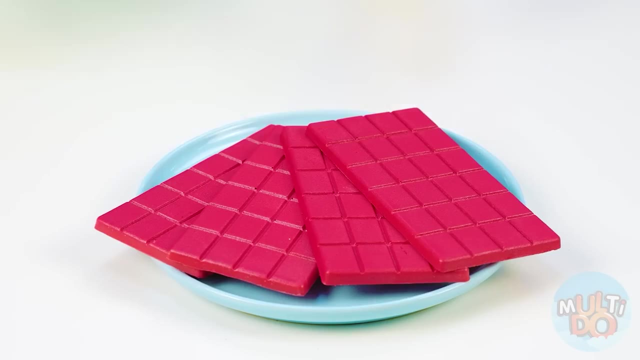 You'll have to eat it anyway. It's enough just to pile a lot of cream. Everyone loves it. Oh, It seems that grandma and Tina cakes are clearly better than mine, But I'll fix it right now. To do this, I need to melt some chocolate. 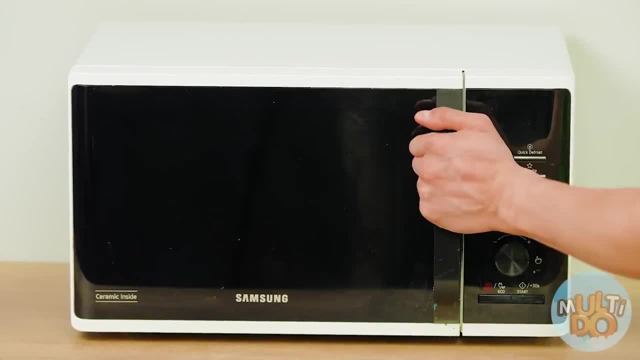 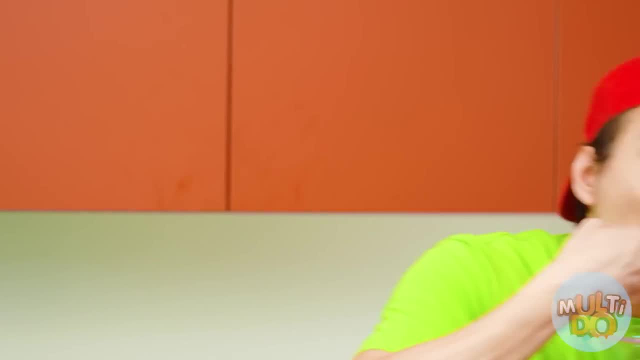 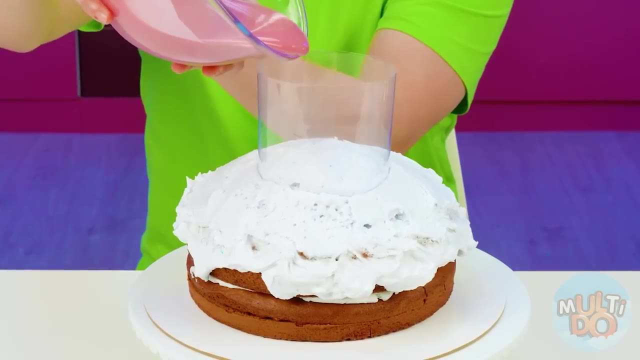 I hope I can do it quickly. Yeah, There it is. Yum, So cool And delicious. It's time to pour this chocolate on this cake, But you need to do this with a special mold. Yeah, don't forget about sprinkles. 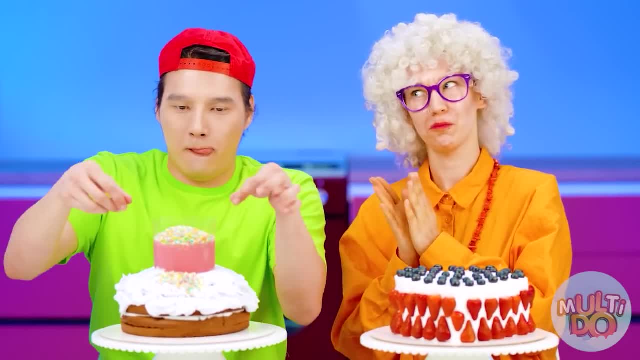 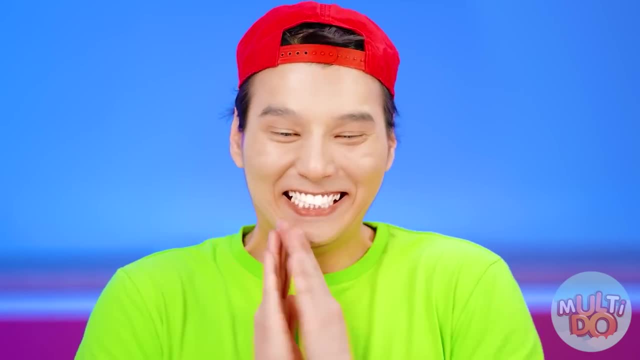 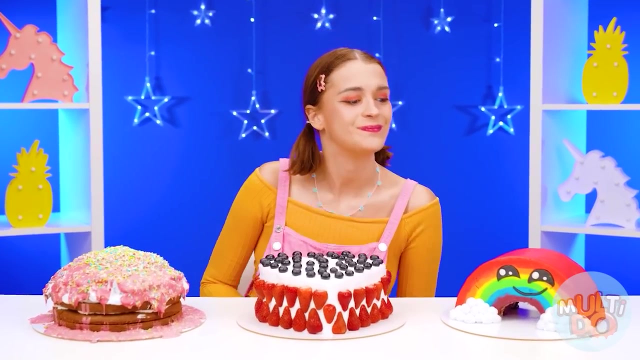 Look at that, Cool, right, And now… Whoa, So cool. Yeah, that's really good, Zack. Yeah, everyone did their best this time for sure. I don't even know where to start, Probably from Tina's cake. 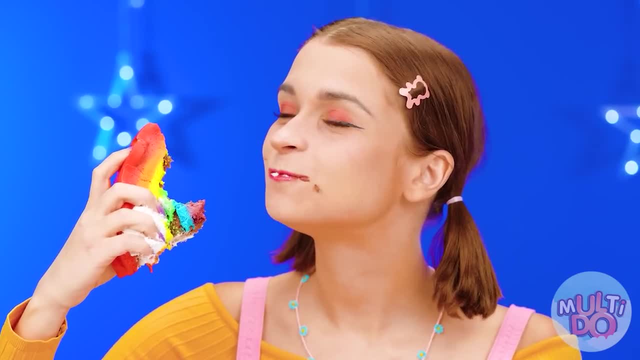 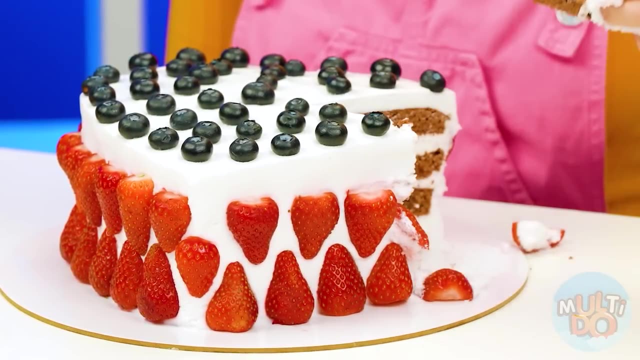 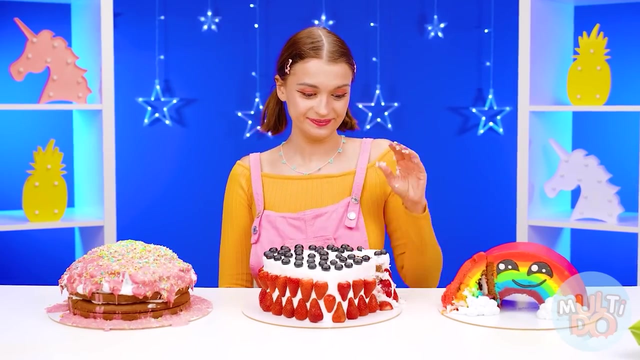 It's so cute, Delicious, but clearly missing something. Grandma, I hope I like your cake more. Mmm, yummy, but there's something missing here. Zack, maybe at least you made the perfect cake Looks, of course, quite ordinary, but the appearance can be deceptive. 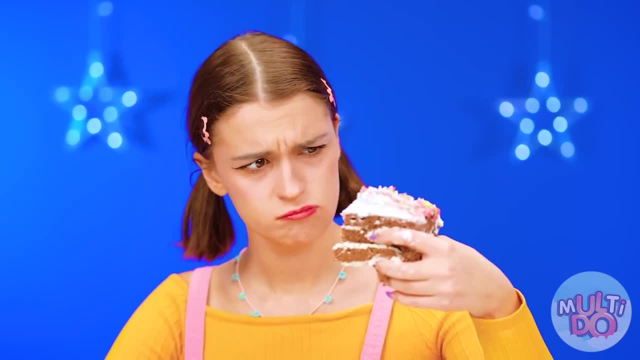 Mmm, smells so good, Mmm, and this is exactly the case. I haven't tasted such a delicious cake before in a long time. Zack, congratulations. this time, the victory is yours, Finally. I already thought I can't win. 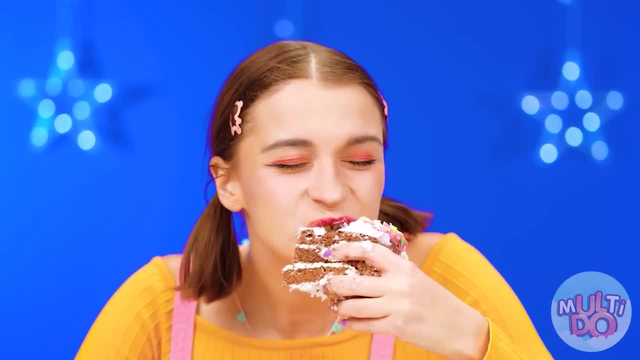 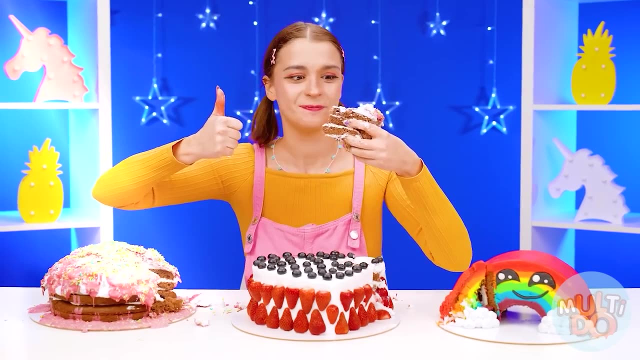 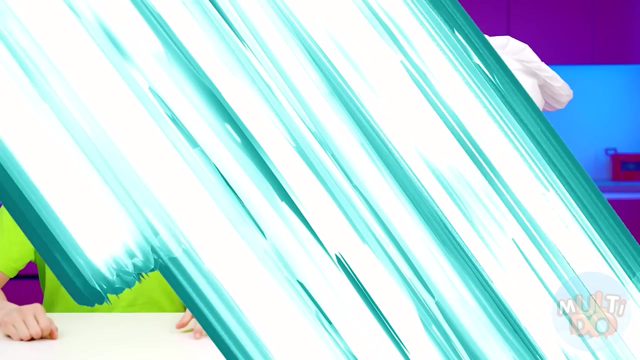